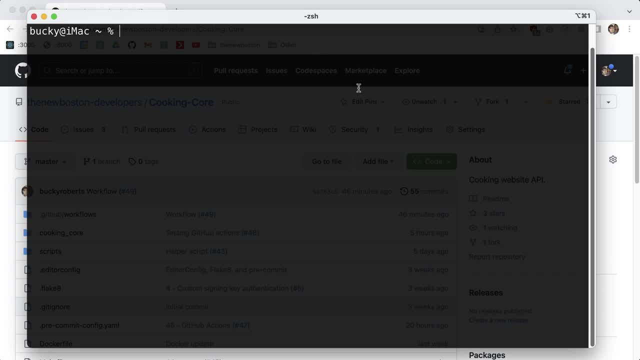 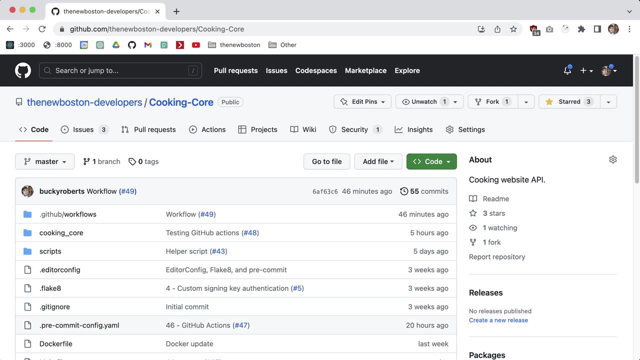 we're going to be doing is I'm first going to make a unique SSH key. Now, with this SSH key, I'm, of course, going to be storing the public key on my server, And for the private key, I'm going to configure it to be stored in GitHub, And what that's going to allow is GitHub, the. 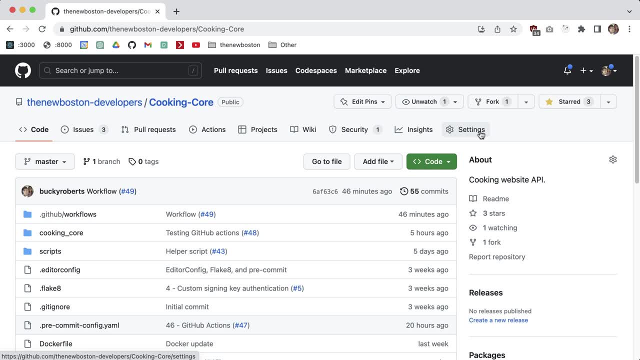 ability to communicate with my server, And once we have that set up then we can go ahead and make a workflow to deploy everything, But pretty much set up the communication first and then get into the good stuff. So whenever you create a new SSH key, 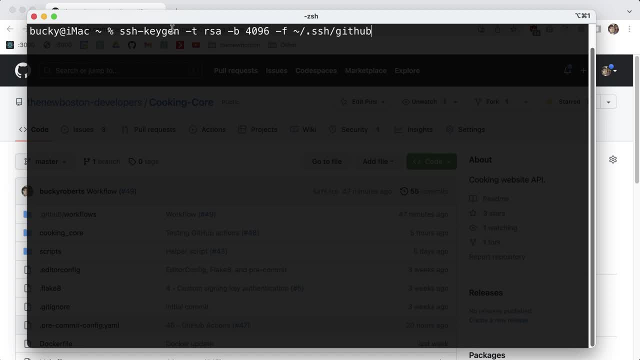 I'll show you the command right here. So pretty much saying that we want to generate a new SSH key. These are just some of the settings for it And the file. I don't want to just have it override my default one that I always use, So I'm going to call this SSH GitHub Now, whenever you create. 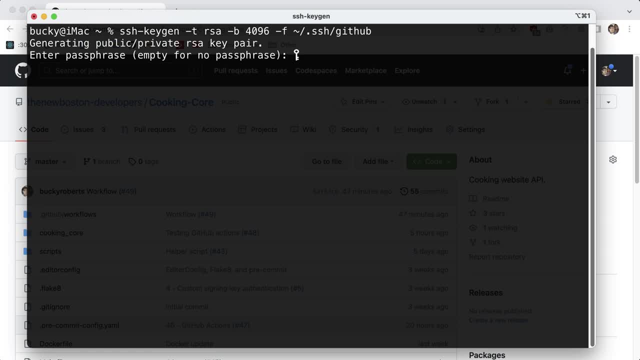 this: make sure not to include a password. If you include a password, then well, your automation is going to break because well, it's going to require someone to manually type in a password. So go ahead and just hit enter to use a blank password or no password, however you want to. 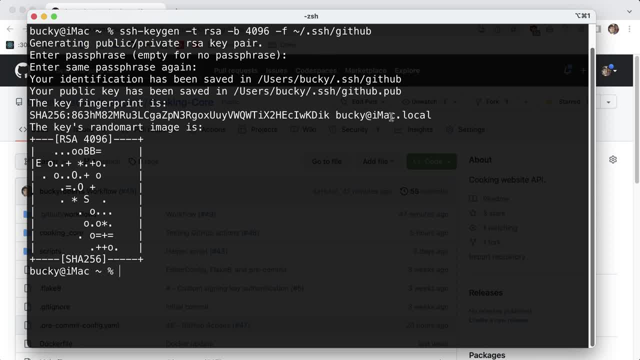 call it, Enter again And there you go. So, as we can see, we now have our SSH key pair created, And this one right here is your private key, And this one right here is the public key That's going to be stored on the server, So it doesn't really matter the order that we do this. 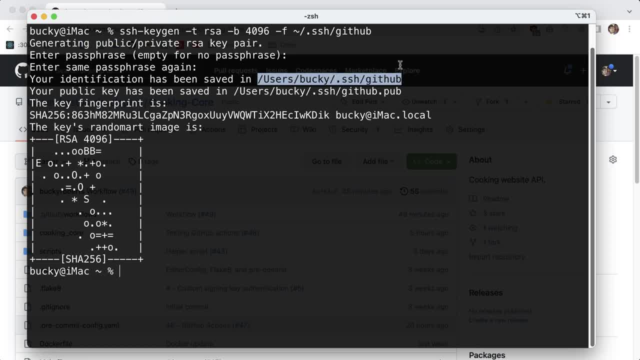 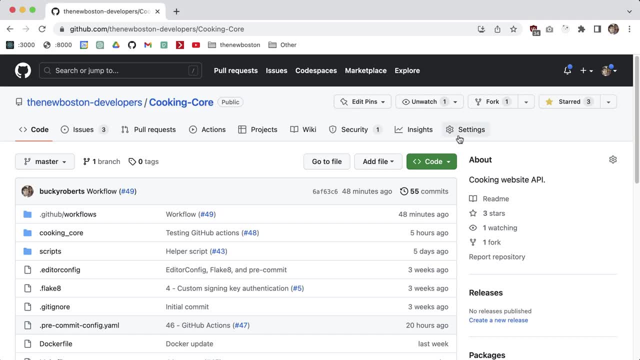 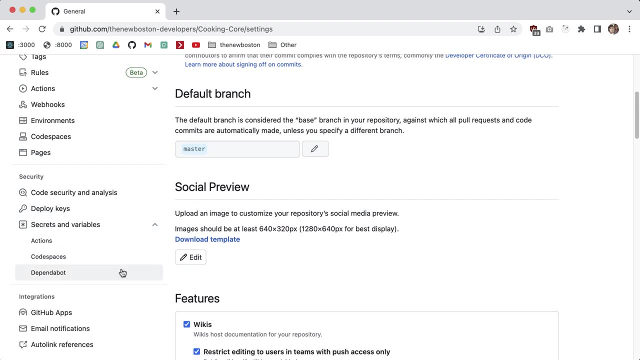 in. but let's go ahead and first might as well just set up GitHub to store this private key. So how do we do that? Well, in our settings, what we can do is scroll down here to go to secrets and variables and click on actions right here, And we're just going to make a new. 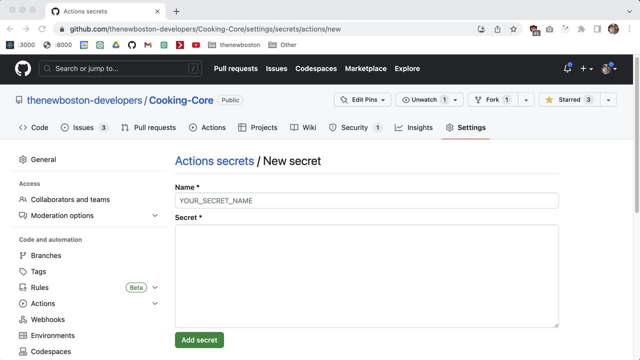 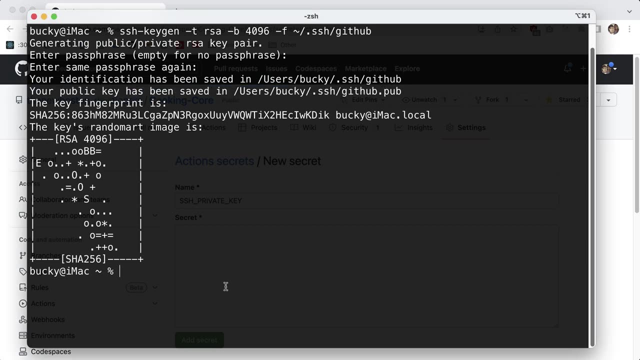 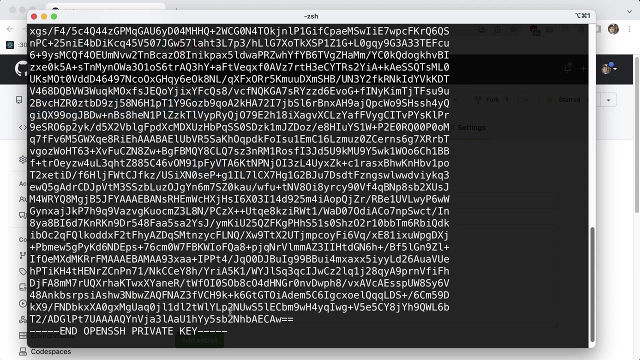 repository secret. So the name of this secret, I'm just going to name it very clear- SSH private key. And for the actual value of this, what we can do is we can just cat out this. So here I can clear this. So cat this and there you go. And, by the way, even though 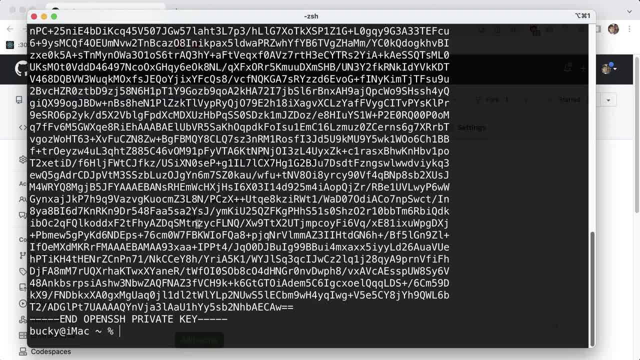 what just got logged out. it says beginning, and then it has your key and then an end. Make sure you don't forget that. So let's go ahead and hit enter, And there you go. Make sure that you actually include these lines right here. 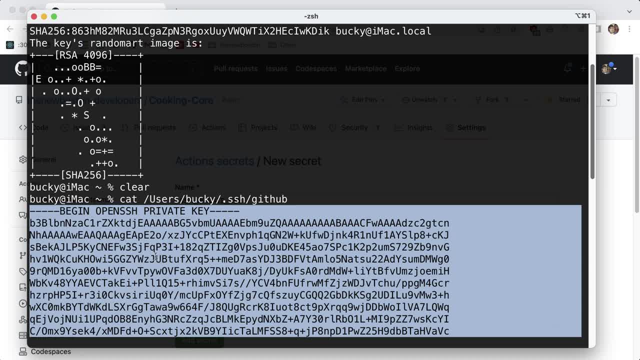 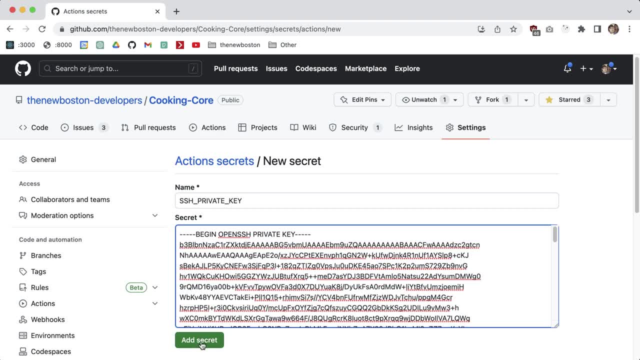 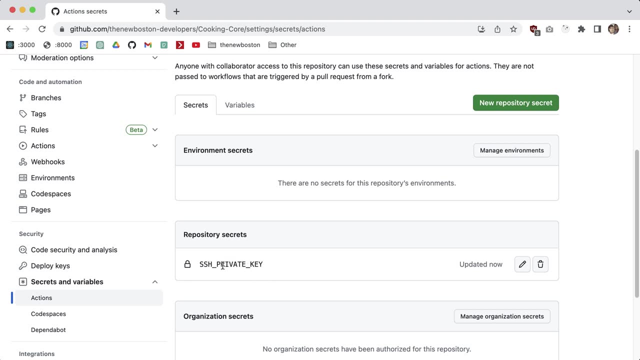 Not just the stuff in the middle, but the actual line that says beginning and end. So I'm just going to copy this and paste that bad boy right in there. Beautiful, Add secrets. And now we can reference in our workflow this private key by using SSH private. 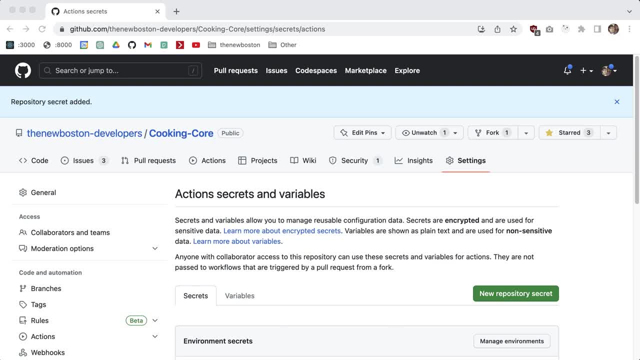 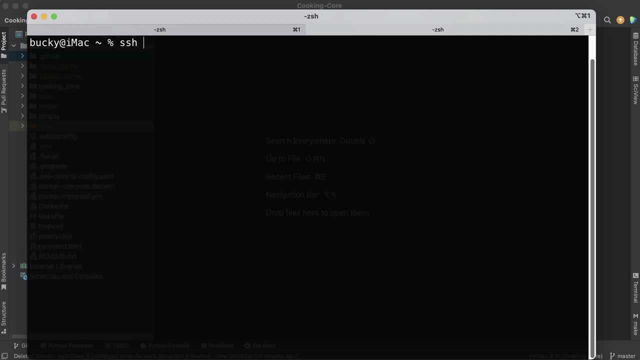 key. So now that this is taken care of, what I can do is I'm going to go ahead and paste this into my server. Let me just go ahead and do this in a new tab. I'm going to SSH into my server. 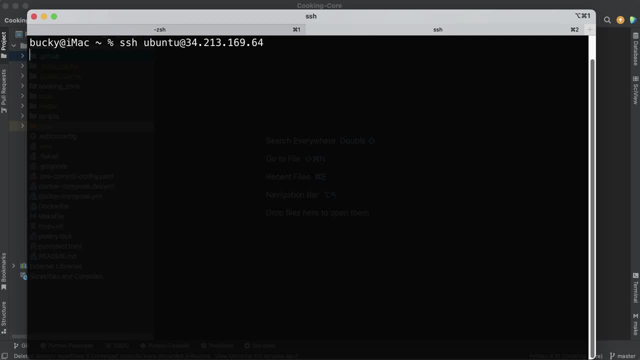 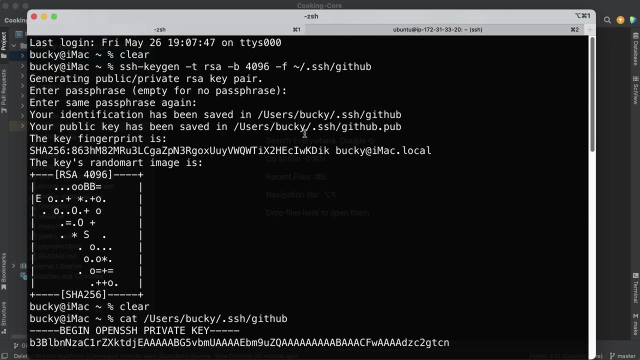 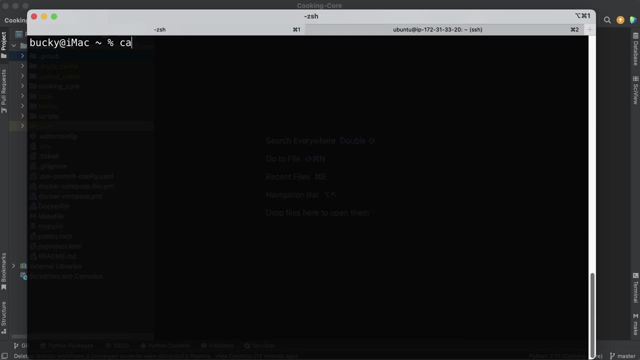 Ubuntu at. and that's my IP, And all right. So what I actually want to do is just cat out this public key, because we're going to be using that in just a second. So let me clear my screen and log this out. So this is my public key. I'm going to go ahead and paste this into my server And that's my IP And all right. So what I actually want to do is just cat out this public key, because we're going to be using that in just a second. 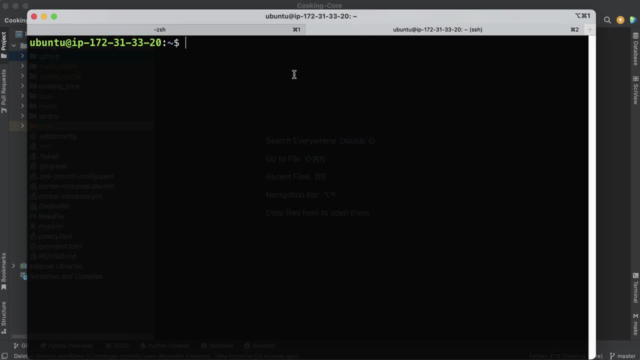 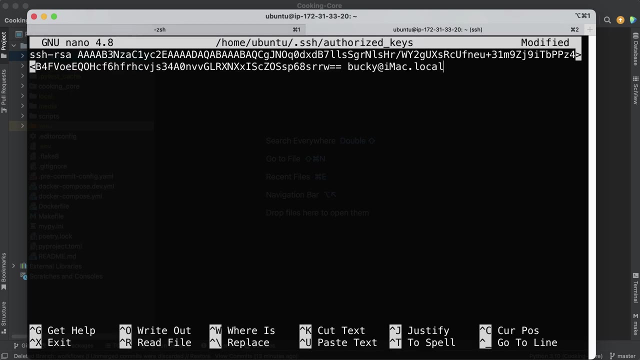 So let me go ahead and copy that Now to add this to my server. what I do is I'll just use nano, sudo, nano, And it is in SSH in authorized keys, And that's the one that I use by default. So right under here I'm just going to paste that new one in and save the file. 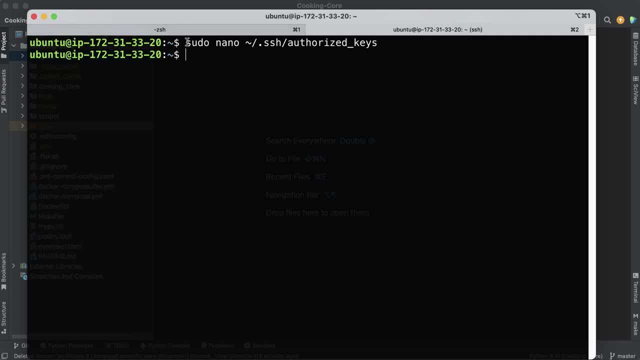 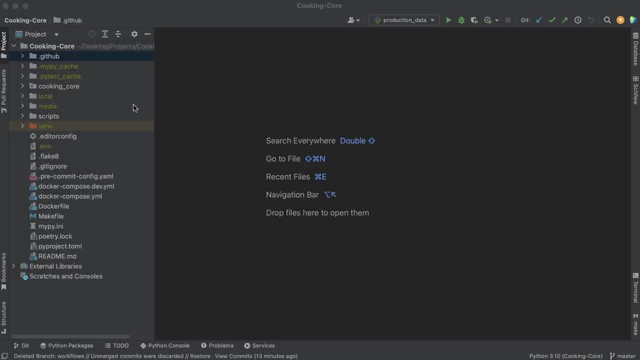 So now my public key is on my server And I believe we can just close this out now. Clear this And yeah, pretty much good to go. So before we actually write this workflow, there are two other little things that I need to do. 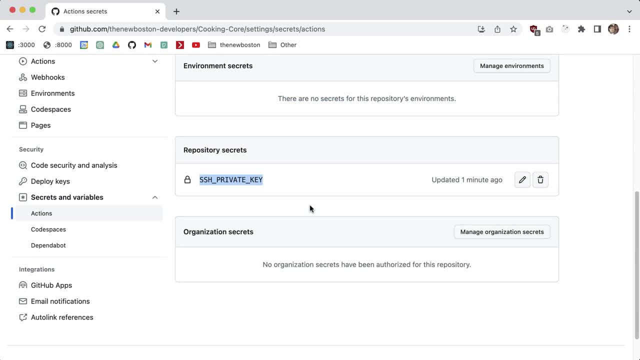 Let me pop open GitHub again. Click the right thing, All right. So you know how we just added this private key right here. What I also want to do is I want to add two more secret values, One for the host, In other words. well, I might as well just do it. 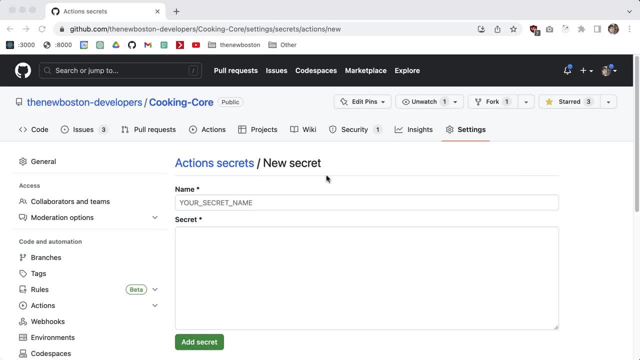 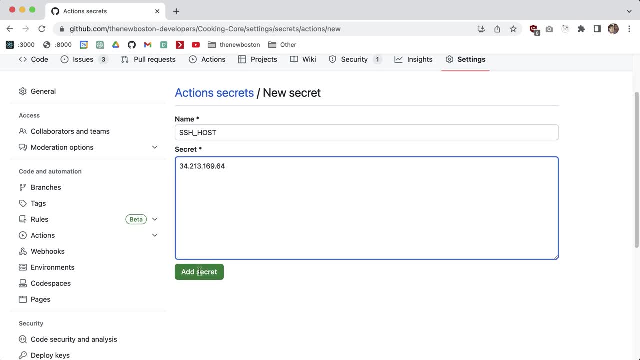 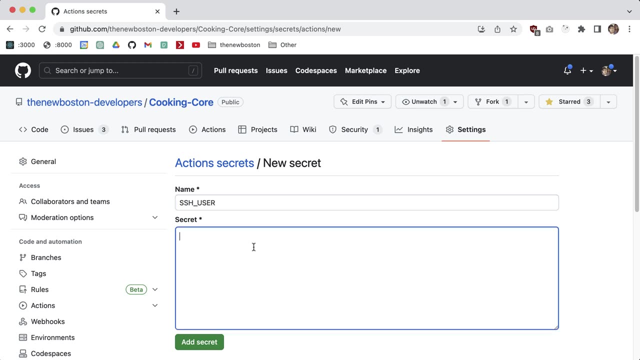 It's probably easier that way. So I'm going to create a new secret, A secret, And this is SSH host, And for this I am just going to give it my IP. And then I'm going to create one more, And this is SSH user, And this is just the user to log in. 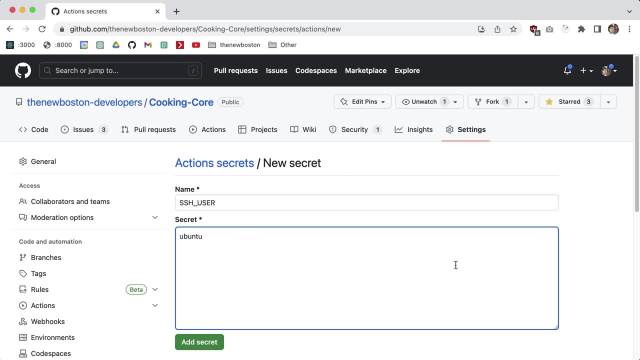 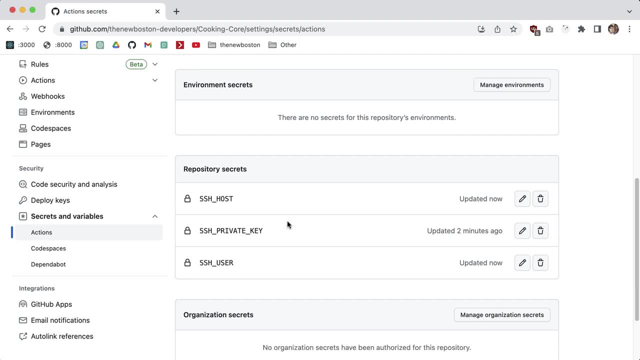 So whenever I log in, I said SSH, Ubuntu at that IP address, And this way I can just use variables instead. All right, So now we got all of our secrets configured And, yeah, I think we are ready to start writing this workflow. 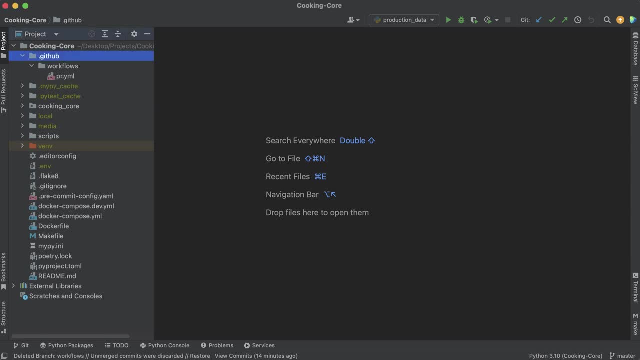 So how do we do this? Well, remember, in workflows. what I can do is, since this workflow is going to be triggered whenever I merge code into master, I'm just going to create a new file called masteryaml, Just like that. And for the name of this I am going to say continuous integration. 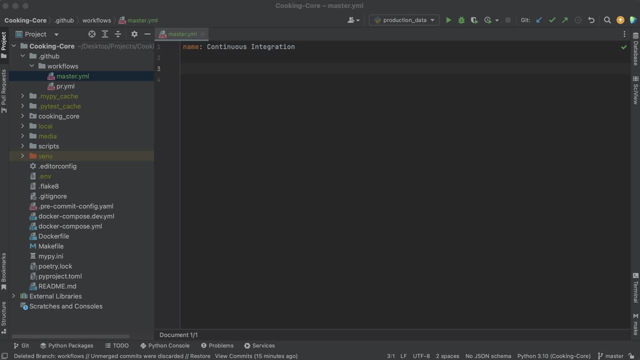 Now, unlike before, where we triggered this on pull request, I just previously triggered it on a personal file called xmmaster. Now you need to remember in a original code this is just going to trigger a new file called Actually on Pusher. 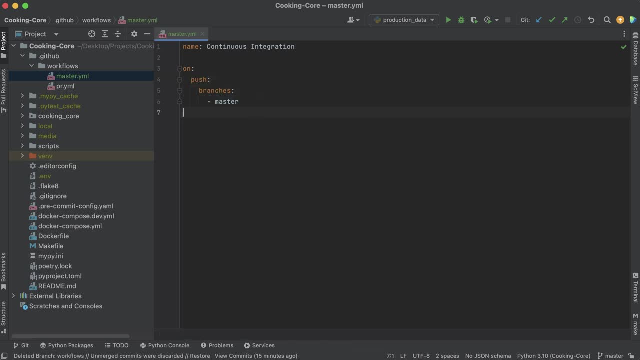 at this point in time in a actually particular code it wasn't- I don't even really have to explain it- Kind of self explanatory on pushes to the branch master. So anytime we merge code in master, this workflow is going to get triggered. 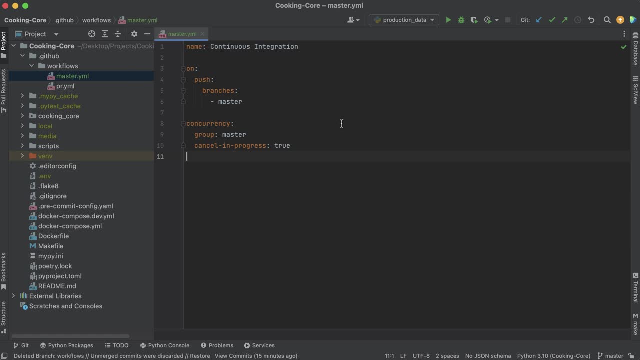 Now, another thing that I want to do- let me paste this in first- is what this is basically saying. let's say that right after that, you made another merge into master, like right again. well, in this case we don't want, like these, two separate processes deploying code at the same time. 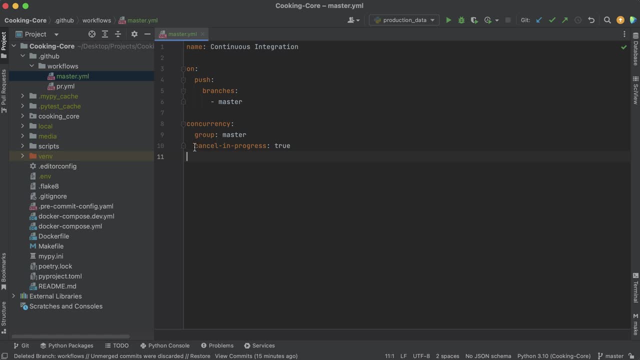 so what this says is: if there's any of these workflows already in progress, then just go ahead and cancel that, and that way the second one is the one that actually gets deployed. so in other words, it pretty much makes sure that only one of these workflows can run at a time, even if you do two. 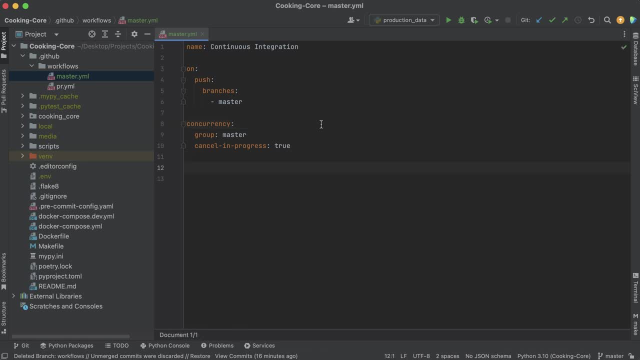 merges right after each other. now for the jobs. unlike before, where we only had one job, which was the quality assurance, here we are going to break up this workflow into two separate jobs. now, the first job is going to be that quality assurance job. in other words, it's going to be: 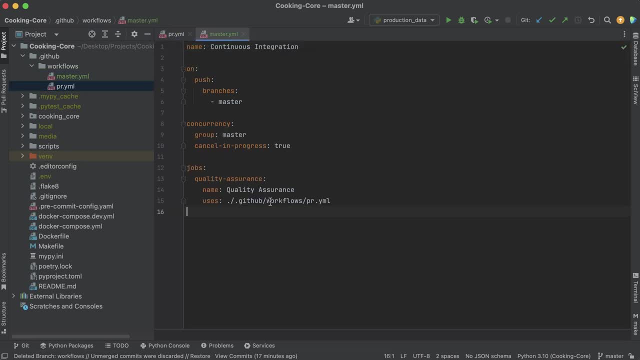 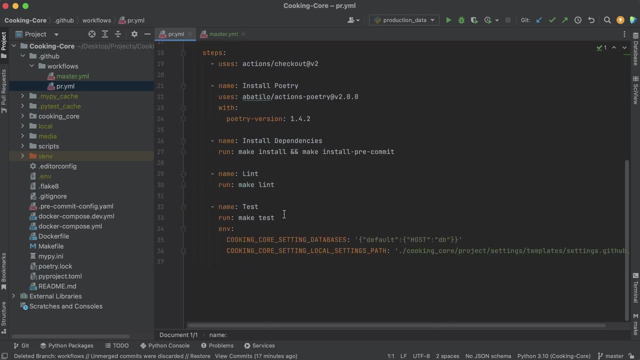 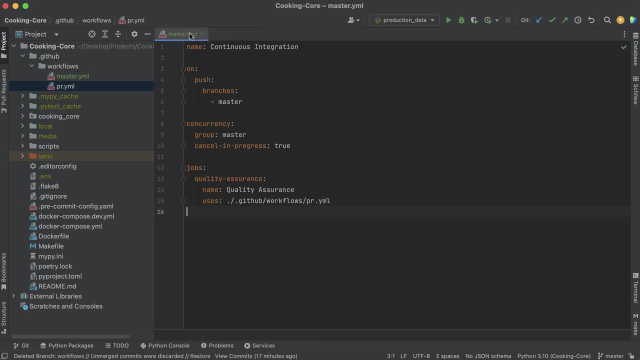 this workflow because before we deploy any code, what we want to do is we want to run this again, like I said in the last video, just to double-check and make sure that our code is properly linted and properly tested. so, before anything happens, it's first going to run this workflow and again, this is how you run other. 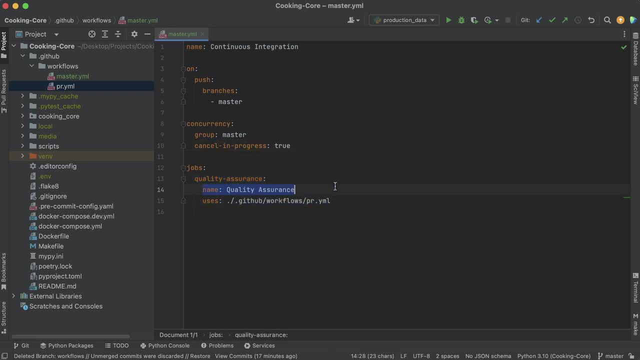 workflows within a workflow. pretty much just give it a name and say uses, and then passed them the workflow and then after this, which hopefully this workflow passes. after this we are going to write one more job, which is our deployment process. so we are just going to give it the name deploy and this needs keyword, is going to reference. 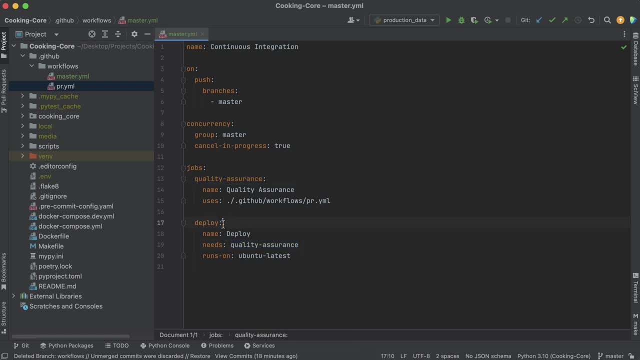 this job right here. so this is pretty much saying that unless this passed, then don't continue. in other words, we need this to succeed before we can deploy. now for this deployment process, we are going to be setting up, of course, the commands to actually like ssh in and do some other stuff, like 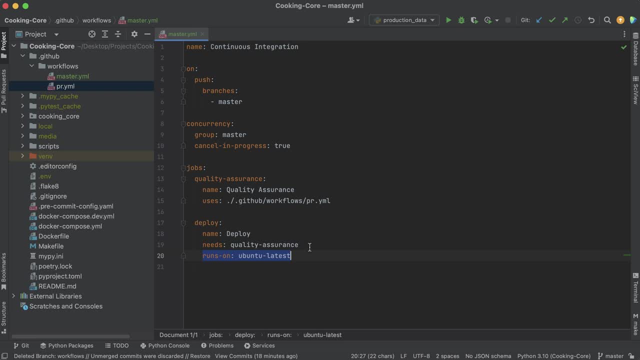 deploy the code, and for this we can just run it on in a butu environment. and what exactly do we want to do in this environment? well, this process is going to consist of two separate steps. the first step is configuring just our ssh. make sure that we have everything set up to connect. 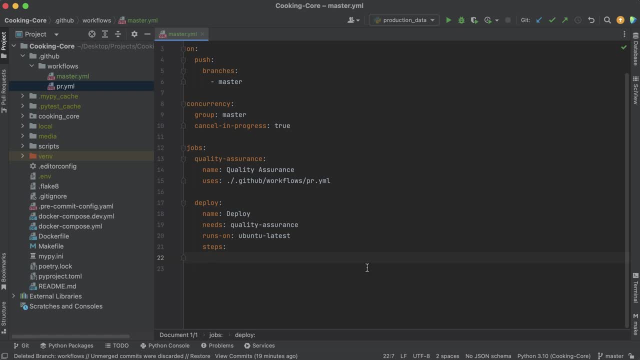 and then the second step is actually running to the command to deploy and update the code, and what this means is we are going to change into the directory where our app's at. we're going to take down whatever's running with docker. compose down, we're going to. 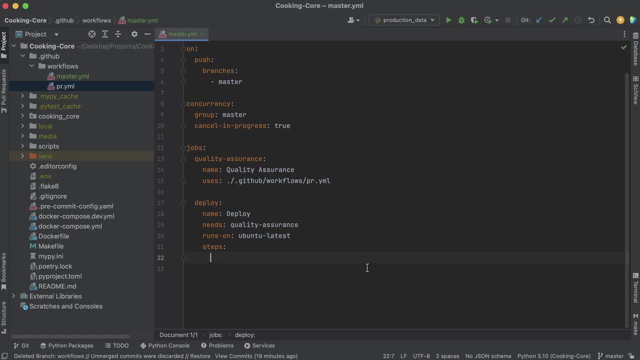 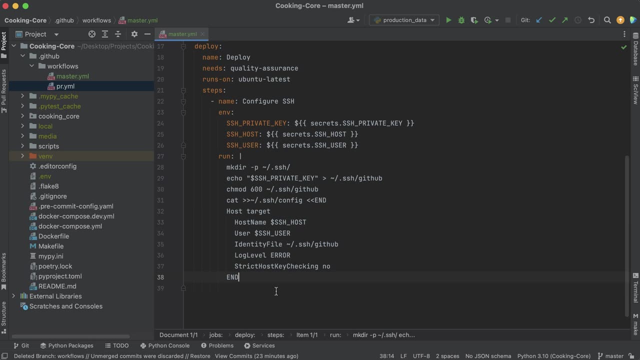 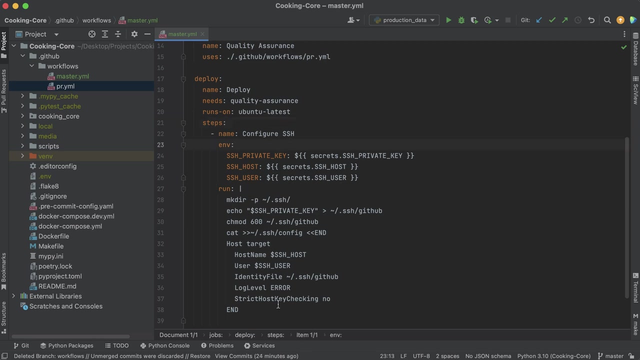 pull the latest updates and then we pretty much just rebuild and spin everything up again. so for the first step of configuring ssh, let me paste this in and then i'll kind of talk you through everything. so the name we're just going to call it: configure ssh. now what we need to do: 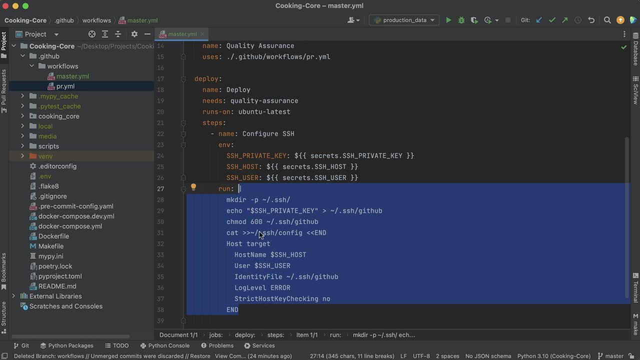 is, we're eventually going to be running this command, and i'll talk you through what this does in a second. however, this command is going to require environment variables, so in order to get these environment variables, what we can do in the easiest way is just to reference the value. 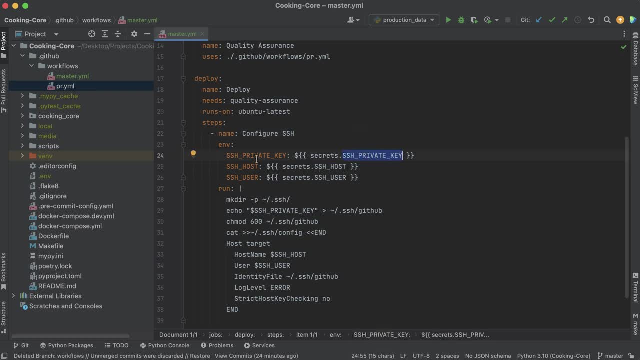 that's stored in github and whatever that value is, just map it over to an environment variable with the exact same name. so this is pretty much taking a github secret and converting it to an variable that we can use in our commands and then, once we have those environment, 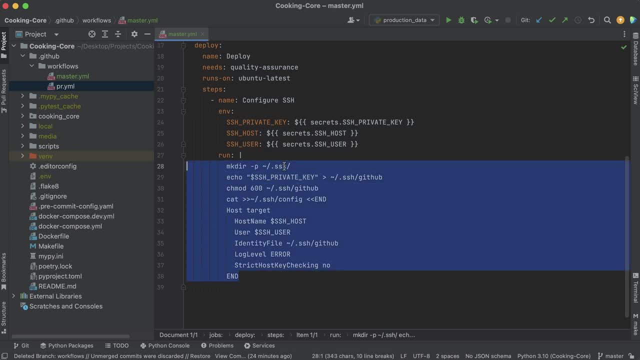 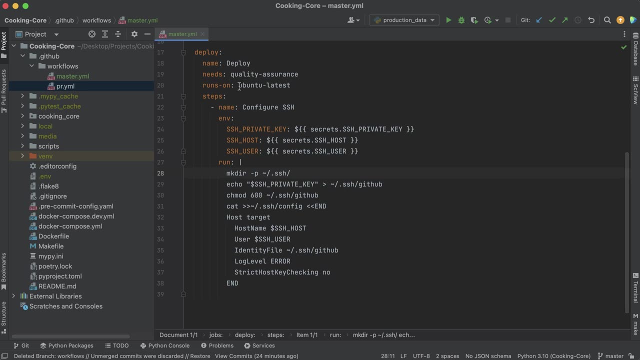 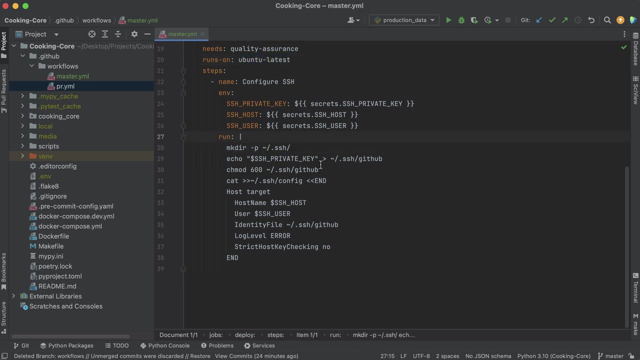 variables that we can use. we're just going to run this command right here, so this is actually multiple commands. but what this is doing is first- and remember, this is all happening basically in a blank version of Ubuntu. so we're first going to make this SSH directory, since that's just where the private keys go. 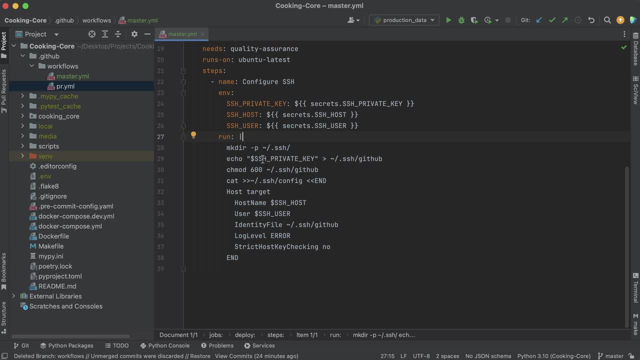 and then, once we have that directory made, we're just gonna take the value of whatever was in this environment variable and stick it in this file right here, which is SSH, github. in other words, we're just creating our sign-in key file. now this line is just changing the permissions of that sign. 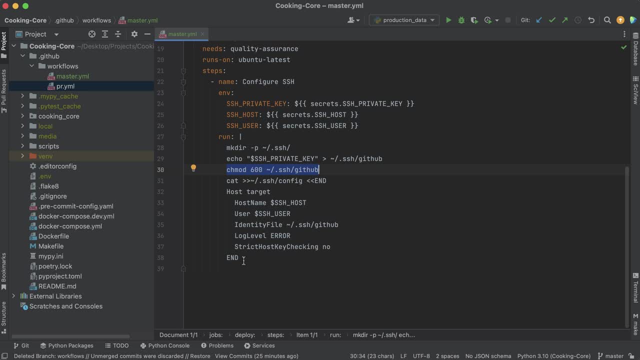 in key file. and then, last but not least, we are running this command right here. so this is a little bit strange if you've never seen that synth X. but basically what we're doing is we are marking the beginning and the end of this bit of code which is pretty much saying we are making a new host called 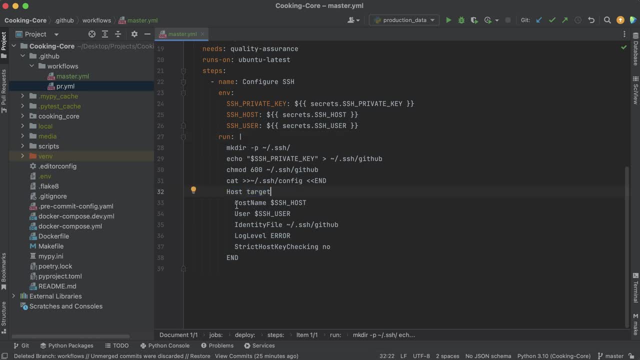 target and this host is pretty much our servers address. this is going to be the IP of our server, the user. this is going to be a boot to the identity file, in other words, the sign-in key that they're going to use. is that one that we just created right here or not? the sign-in key, the private? 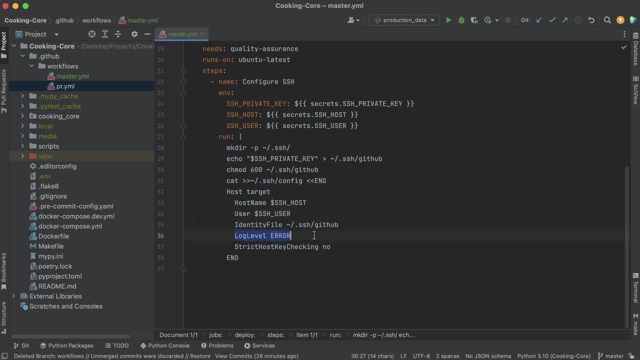 key, thinking of my app logic, the log level- just log out any errors- and the strict host key checking. you know, whenever you first SSH into a server and it says, hey, the server identity, yada, yada, and you got to manually type yes, well, what this does is it just says: hey, don't worry about that, I, we're not, don't. 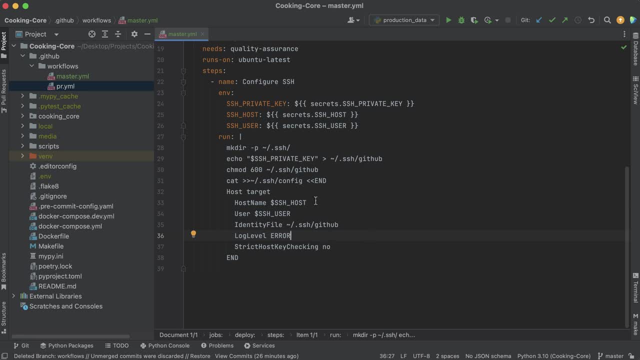 bother us with having to type anything. just go ahead and you know, skip that part. so anyways, this pretty much just configures the where we want to log in and how we're going to log in, and then, with this bit of code right here, we're going to cat, or pretty much like display it out, and then this redirect directive. 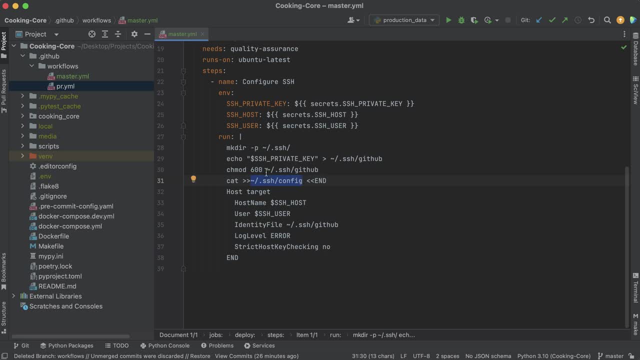 pretty much just sticks it or appends it to this SSH config file. so, in short, we are taking this text and appending it to this file. so now, whenever we SSH into the host target, it's gonna pretty much know exactly what system we want to connect to and how we want to connect. now, with that said, we only need to run one more. 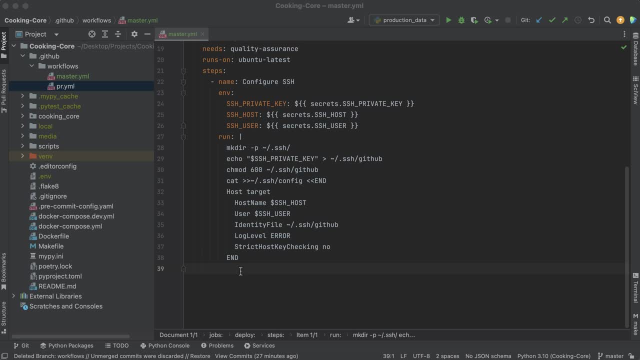 command, let me go ahead and paste it in and that is this command, or this one last step. I should say. so this is just gonna run our actual deployment. and to run our deployment, what we do is we're just going to SSH into this target, and in other words SSH into my ec2 instance, and now, once we're SSH in, we pretty much 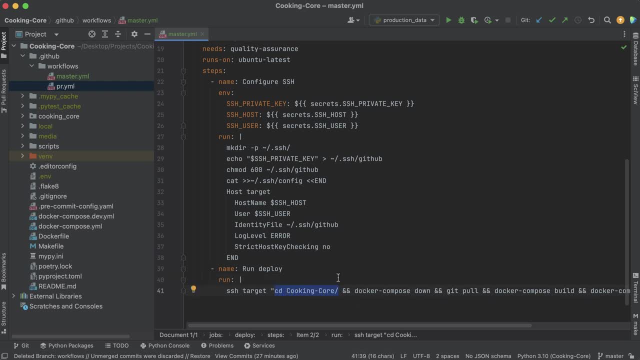 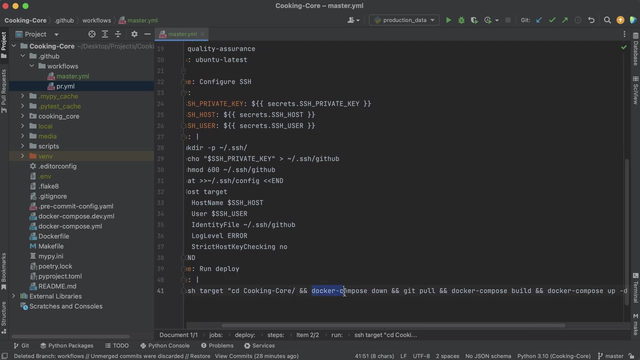 just write the commands that we would normally do if we were- just, like you know, already SSH in there and updating the server. and, of course, to do that, what we need to do is we need to change into the cooking core directory. that's where the app is now. after this, we're gonna run docker, compose down and that's gonna. 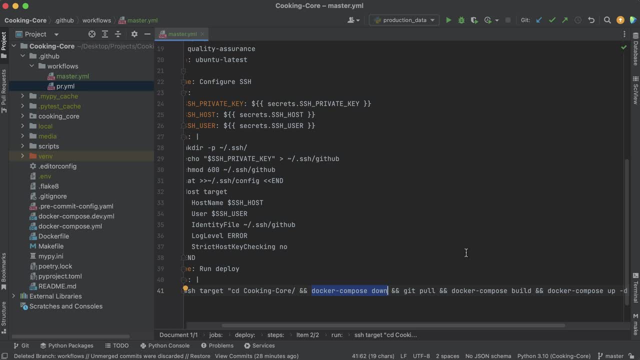 bring down those containers. remember we're gonna have for the database and we have another container that the app runs in. now, once those containers are down, we're gonna pull down the latest code and remember at this point in time everything was already merged into master. so this is. 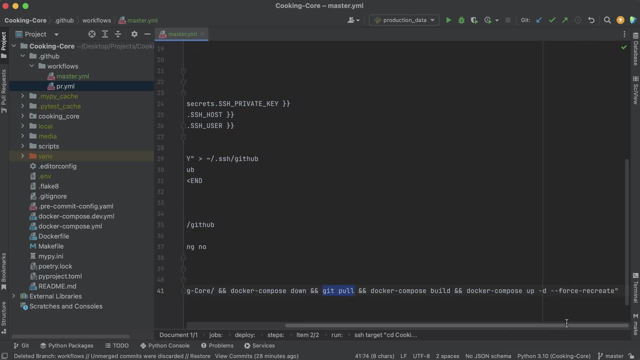 like brand spanking new code, the latest changes that you made to your app, and once we have the latest changes, we're just gonna run docker compose build to rebuild those images with the latest code and then, once we have everything built, then we can go ahead and spin up the. 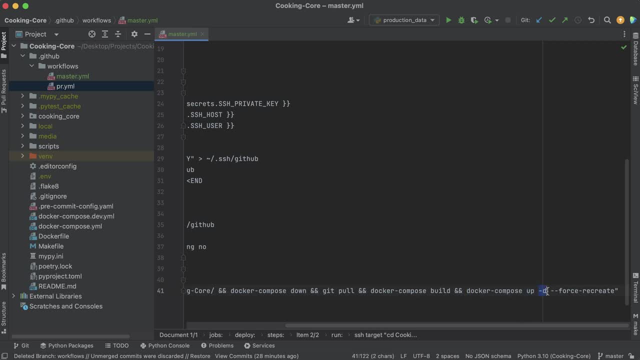 containers using docker, compose up, run it in demon mode and then we're just gonna make sure that we have everything recreated and, yeah, get all the latest stuff. so let me actually just add a blank line to the end of this. and now, as soon as I push this up, since I'm not on any other branch and I'm just pushing- 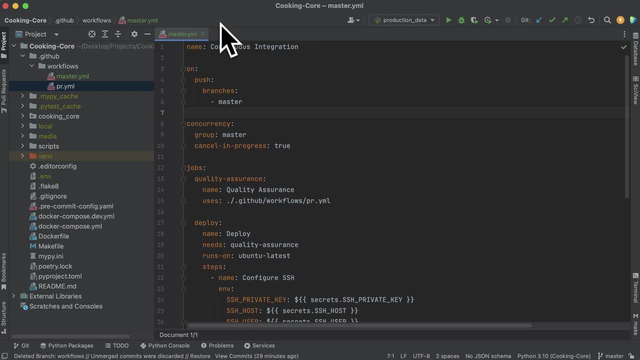 right up to master. this should actually kick off this CI process. so let me just go ahead and push it up and I'm just gonna run docker compose up and I'm just gonna push it up and I'm just pushing right up to master. this should actually kick off this CI process. so let me just go ahead and push it up and I 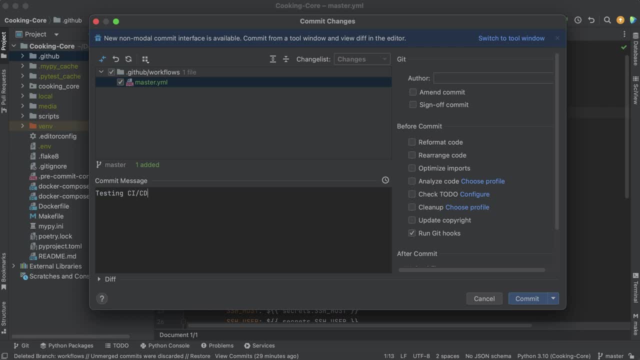 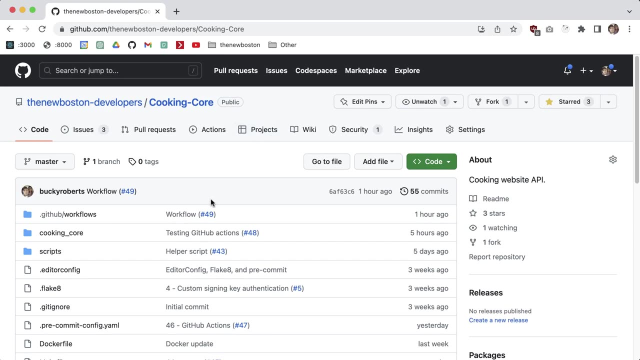 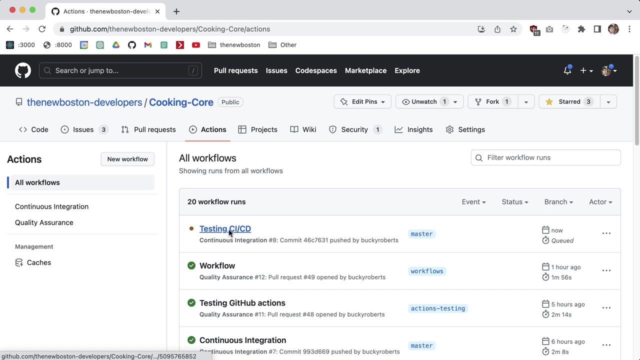 can say testing CI, CD, and let me just commit and push that and check it out. so now let me go in my actions and you can see that, yes, this new workflow is running and I want to view the details of it, so I'm just gonna click into this. 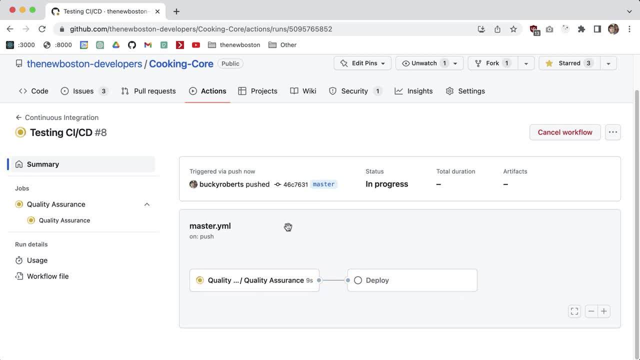 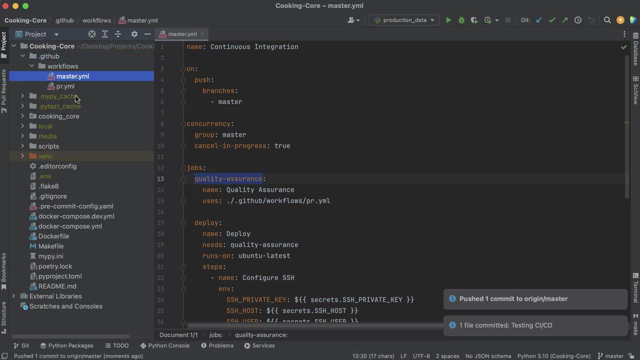 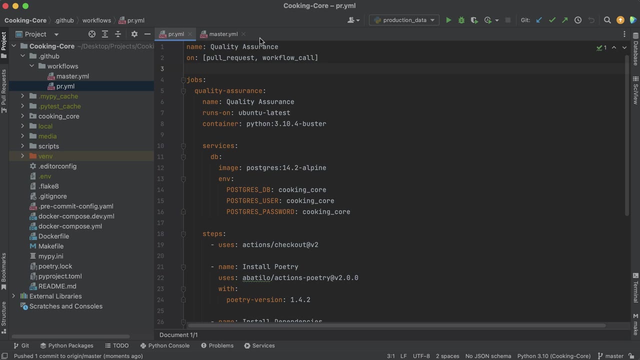 and this is how it's displayed. if you have multiple jobs, so the first job that we have by reference back here is this QA job- what actually references this right here. so it's gonna check all my linting and testing and if that succeeds, then it's gonna go ahead and run this deployment. 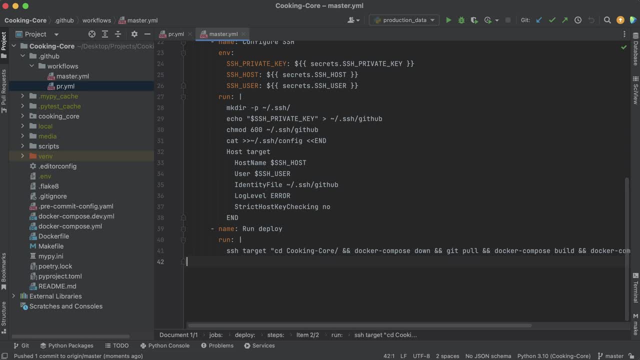 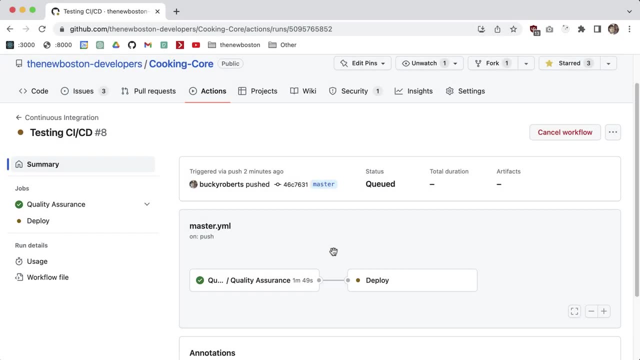 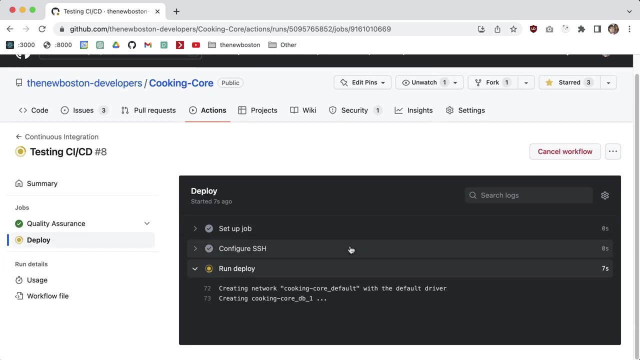 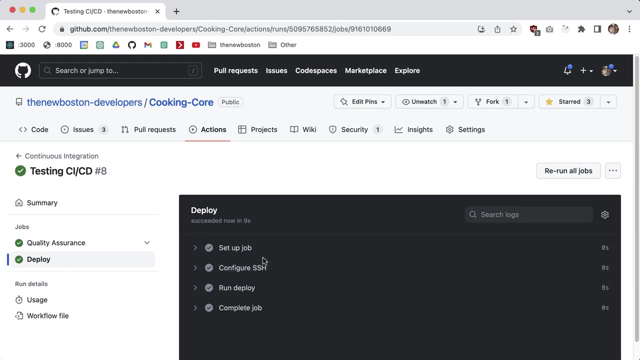 scripts and as long as I didn't mess anything up, it should automatically deploy that. so let me pop this back open. all right, look like everything passed QA. now we can see if our deployment process is working. actually, let me click into this: SSH configured properly, running. deploy- looking good. Wow, pretty quick. so this looks like it was all good to go. 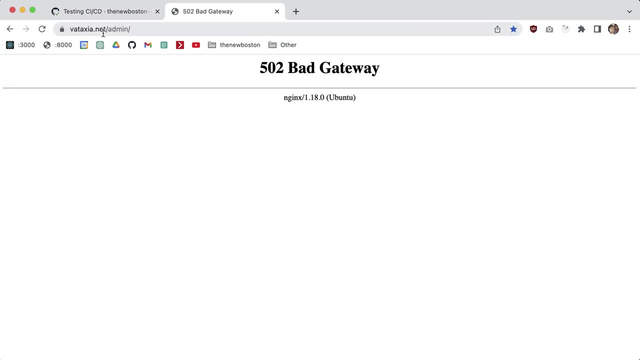 and we can verify that, actually, if we go to Vitaxia NetAdmin. so it looks like we're getting an error. but this is actually good, because, well, errors aren't good. but whenever I update my server, then right after what it does is, it has to, of course, restart docker and restart nginx. so this just means that nginx is. 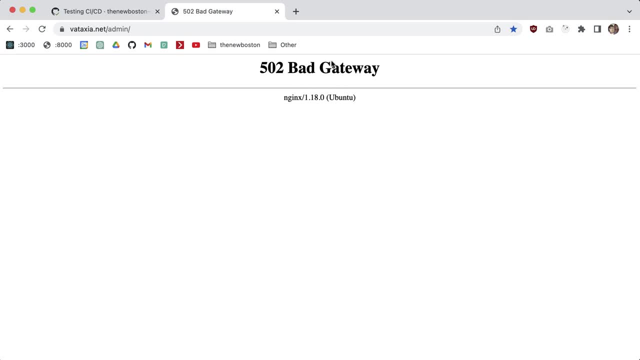 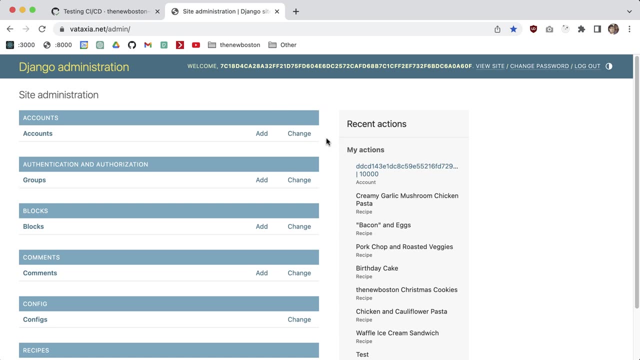 restarting. now the nginx process should restart in like I don't know, 10 seconds or so. so as long as I refresh that, I can see that, yes, everything was deployed and restarted successfully. so that, ladies and gentlemen, is how you set up a very basic CI CD workflow. now another thing that I want to point. 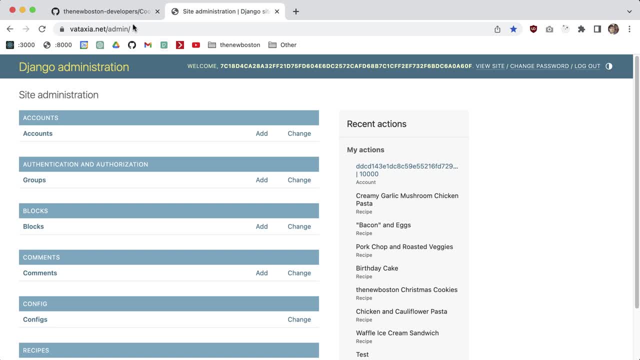 out is that, even though this is indeed a bare-bones working CI CD pipeline, this isn't like the ideal process, and I say that because remember whenever we deployed this, even though I was kind of happy whenever I saw the nginx error, you probably don't want like a production environment throwing these errors and